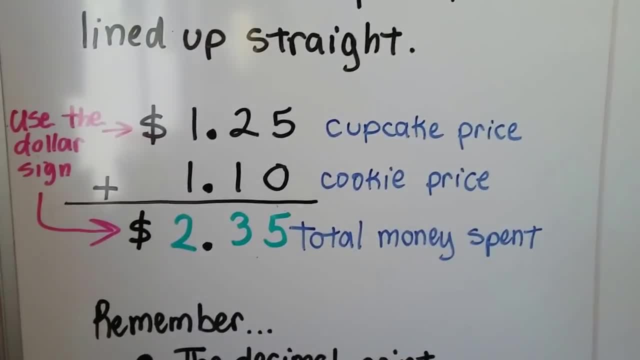 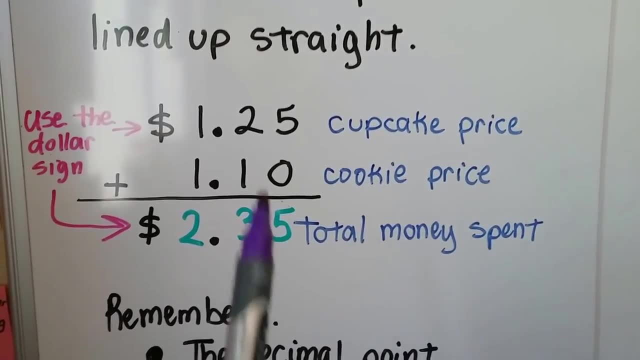 and our decimal points are stacked nice and pretty on top of each other. If we bought a cupcake and a cookie and this was the price of the cupcake and this was the price of the cookie, we could total them, We could add them and find the sum to find out how much money we spent. You have to remember. 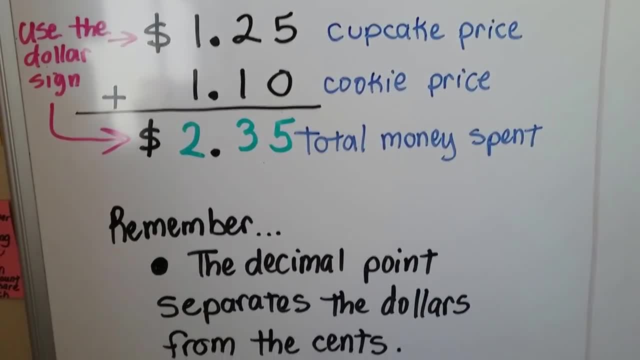 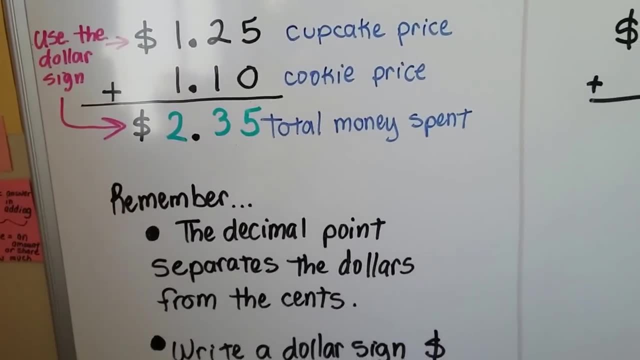 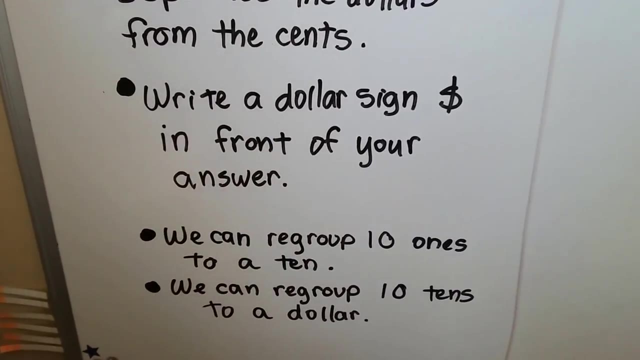 to use a dollar sign when you're adding money. okay, Just remember that the decimal point separates the dollars from the cents. This is the dollar side and that's the cent side. We have to write that dollar sign in front of our answer and remember we can regroup 10 ones to a 10 and 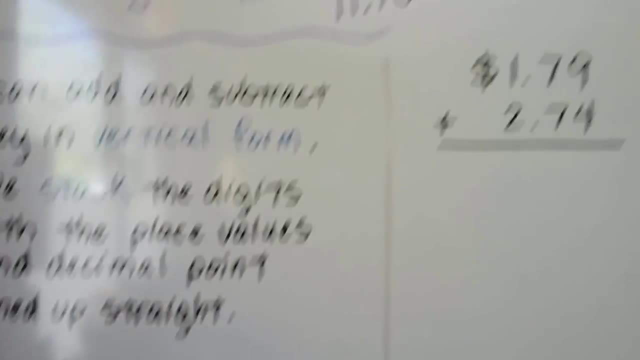 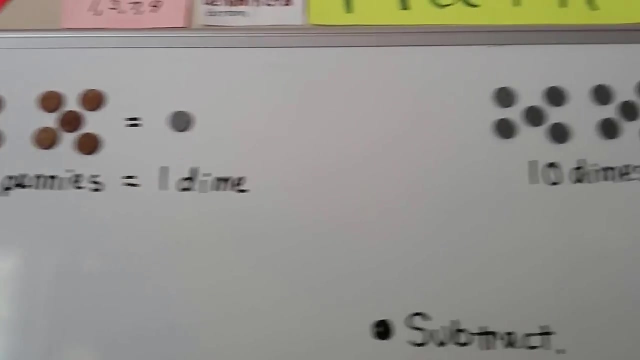 10 tens to a dollar. So remember, 10 pennies equal one dime. right, That's 10 ones and we regroup it as a dime. and when we get 10 dimes, we can regroup it as a dollar, because that's 10 tens, okay? So 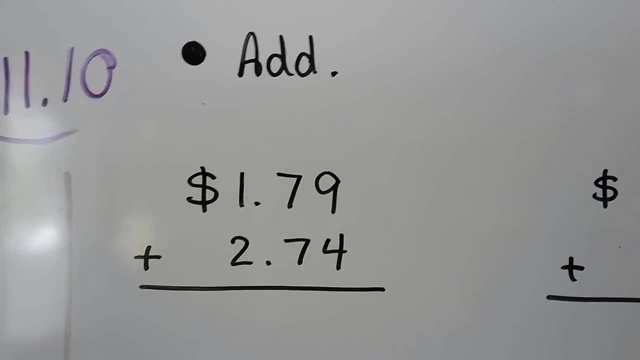 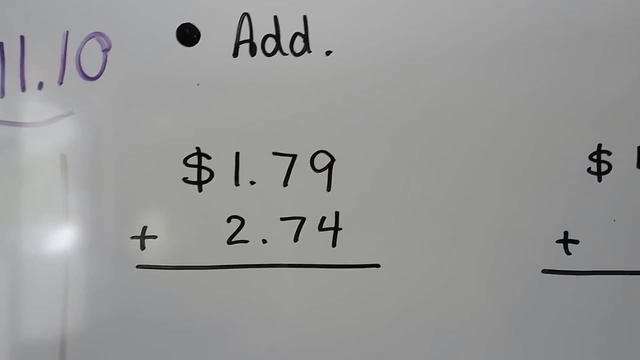 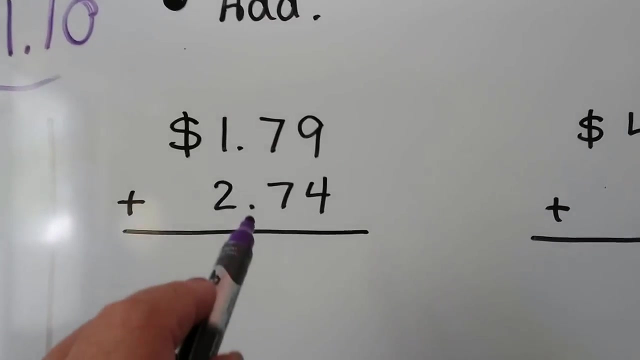 let's see if we can add these, and we're going to follow the same rules as we did adding three digit numbers. We just now have this decimal point and a dollar sign that we have to put in. That's all Same thing as adding 179 plus 274.. We just have to remember there's going to be a decimal point. 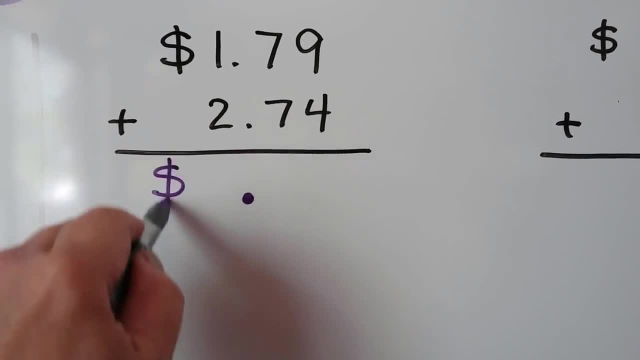 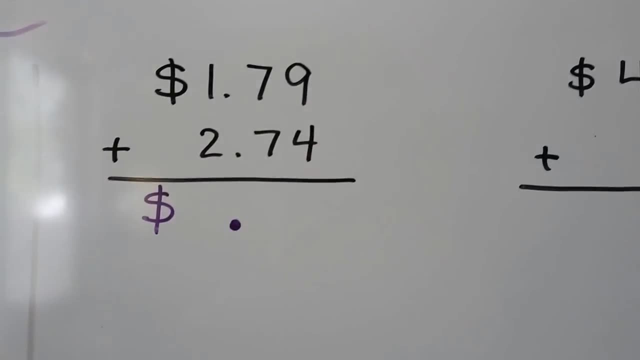 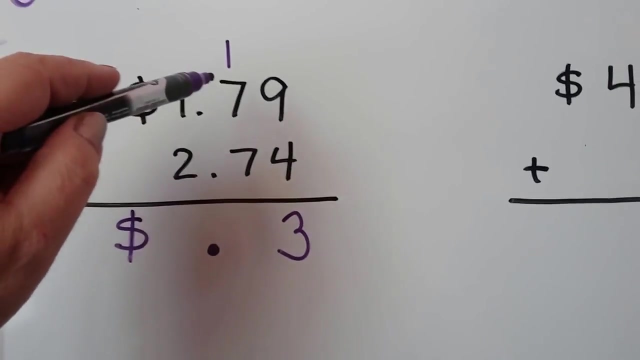 that comes straight down right here and we're going to need a dollar sign. That's the only difference. okay, So let's add the ones place first, like we should. 9 plus 4 is 13.. We need to regroup the 1 and put the 3 down. Now we add the 7 plus 7, because that's a nice double to add, That's. 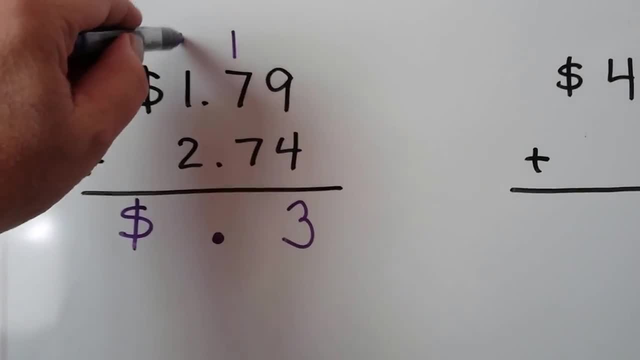 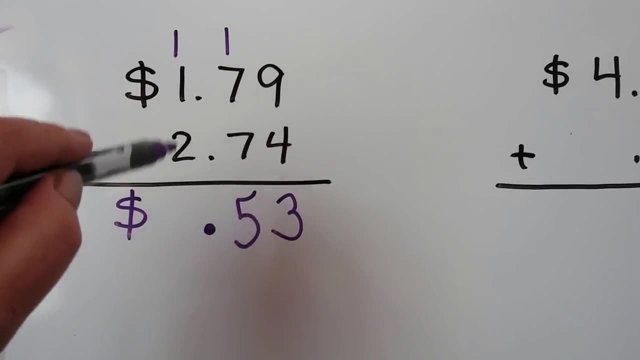 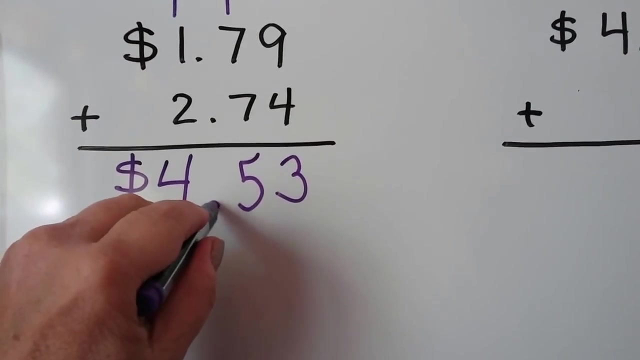 15 and we just regroup just like we would do with hundreds. It goes up into the dollars, See. We add the dollars and we have 2,, 3,, 4.. We have $4.53.. See, Let me move this down to the bottom, where it. 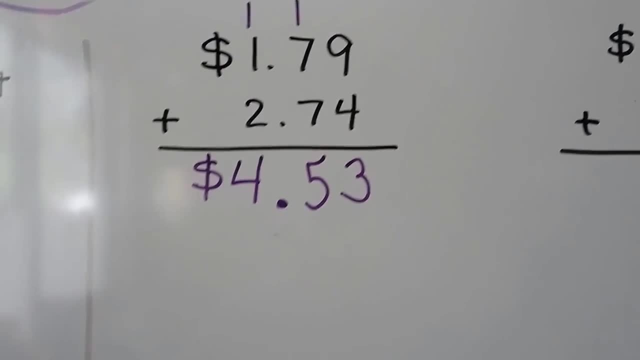 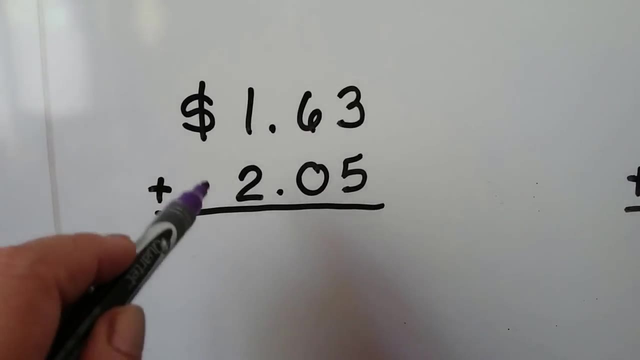 belongs. See, We just have to remember our dollar sign and our decimal point. Let's try this one. We have $1.63 plus $2.05.. Now do you notice there's no dollar sign here? That's because we have to. 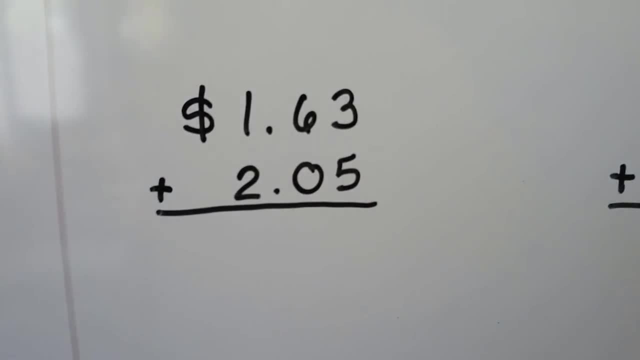 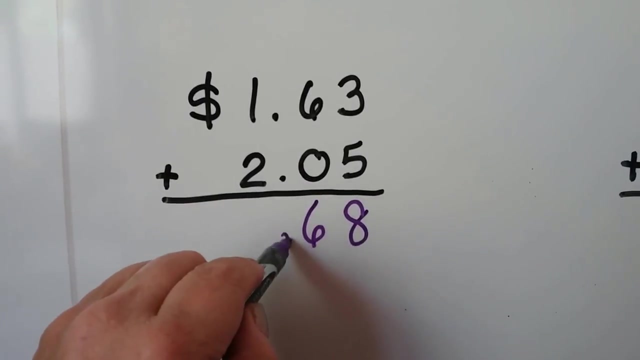 regroup the 1 and put the 3 down. That's because this one is representing both of them. okay, We have the decimal point there, so we know we're adding two amounts of money. Let's add the ones place: 5 plus 3 is 8.. 6 plus 0 is 6.. We put our decimal point nice in a row, See, And then we add: 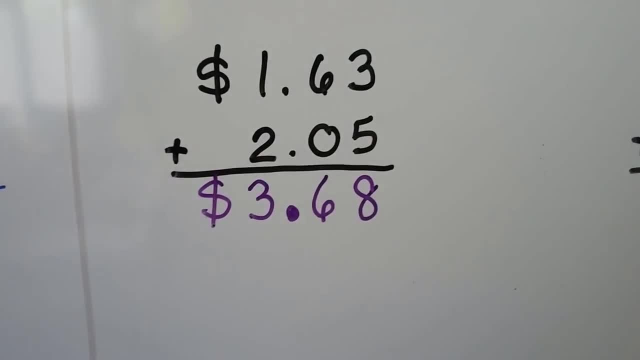 the 1 plus 2, which is 3, and remember our dollar sign: $3.68.. All right, Let's try it again. I'm going to do another addition, one. We're going to add $4.83 with 75 cents. You can write 75 cents. 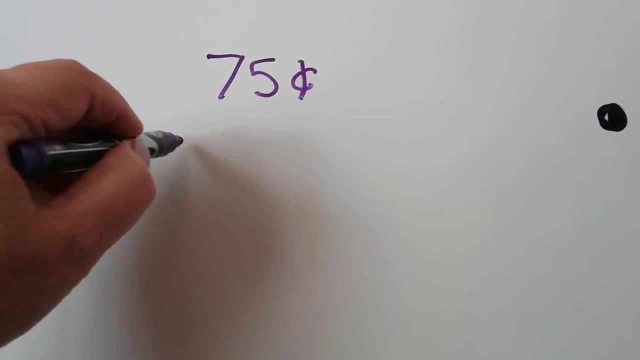 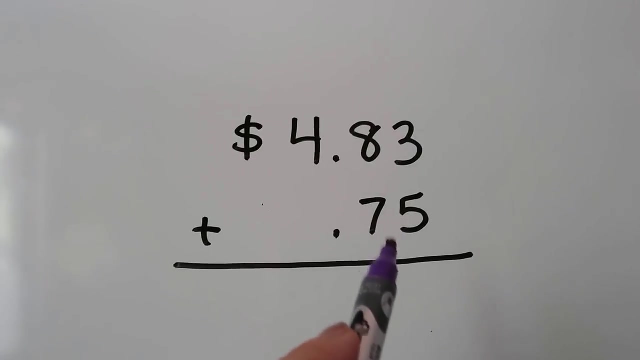 like this, with a cent sign, or we can put .75 to mean 75 cents, because, remember, everything on this side is cents and everything on this side of the decimal point is dollars. So when you see this decimal point and then two numbers, you know it can mean money. All right, 75 cents. So let's add the. 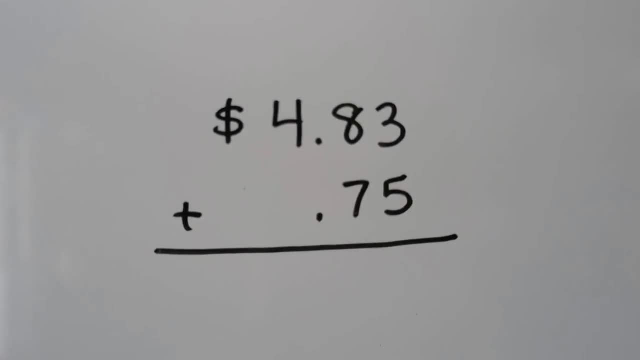 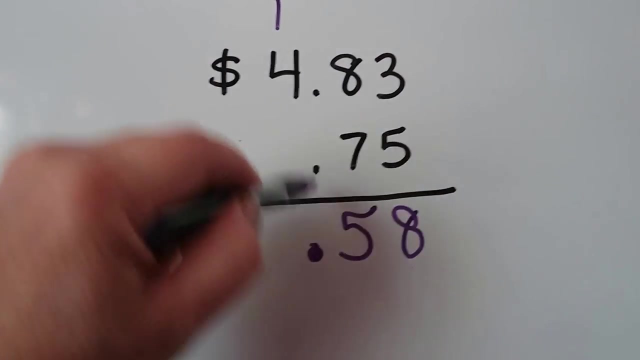 ones place. 5 plus 3 is 5.. 6,, 7, 8.. 8 plus 7 is: do you know? It's 15.. We're going to regroup the 1 and put the 5 down. We're going to put our decimal point in a nice, pretty column coming down. See It matches. 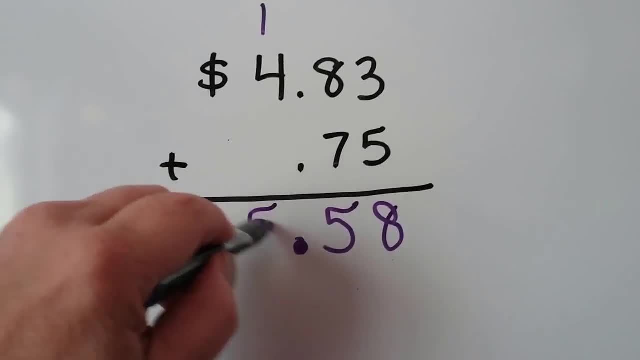 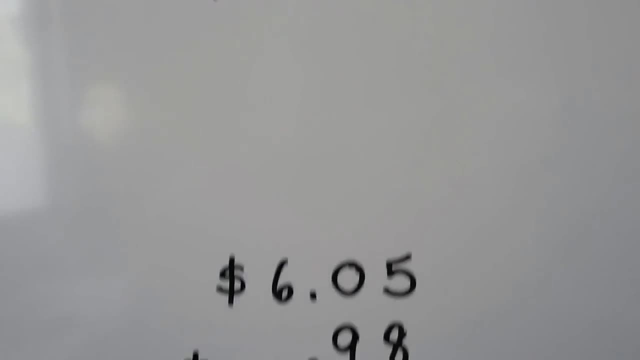 those. Then we're going to add the 4 and the 1 and get a 5.. We're going to remember our dollar sign and we have $5.58.. Let's try it again. We've got $6.05 and we're going to add 98 cents. That's almost another dollar. 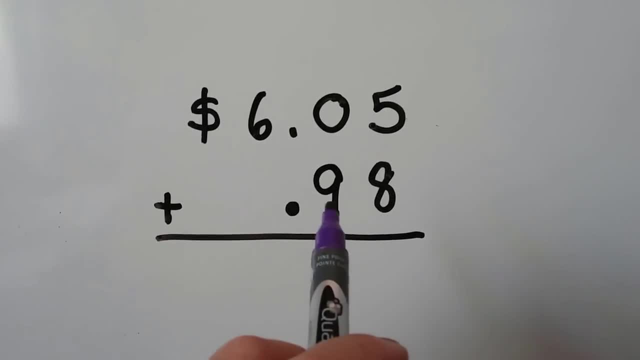 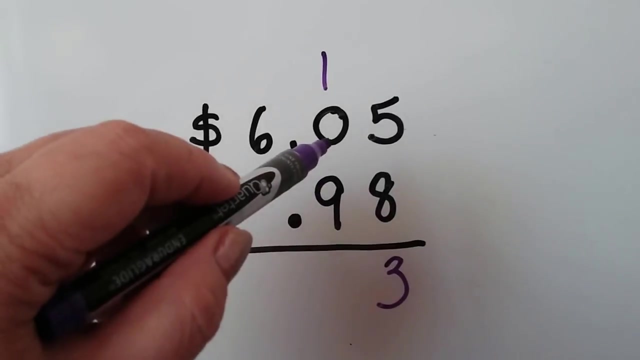 isn't it 98 cents? Because we could go 99,, 100 and we'd be at a dollar, wouldn't we? So it's going to be really close to adding a dollar. We add the ones place: 8 plus 5 is 13.. 9 plus 0 plus 1.. 9 plus 0 is: 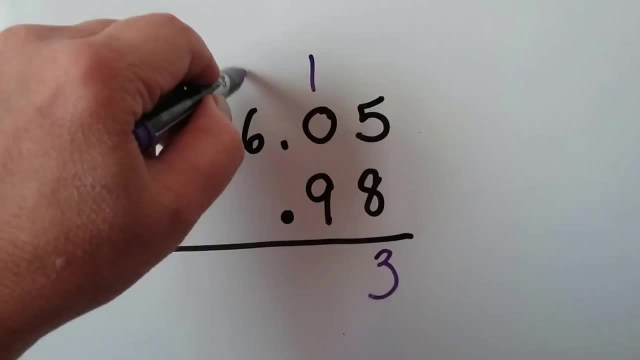 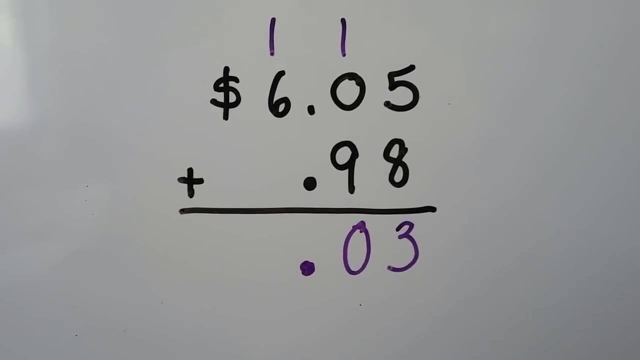 9.. 9 plus 1 more is 10.. We need to regroup again. We need to put the 1 up here and the 0 from the 10 down here. We need to put our decimal point right here in a nice, pretty row column- I'm sorry- in a nice. 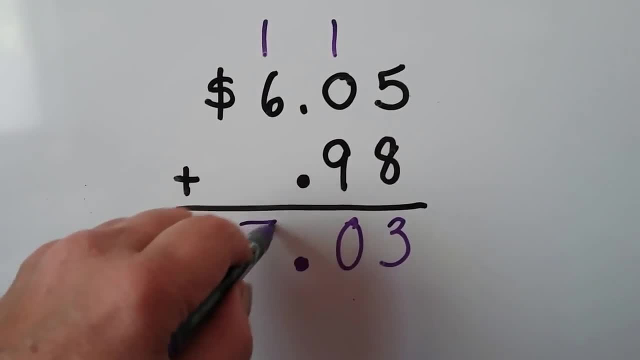 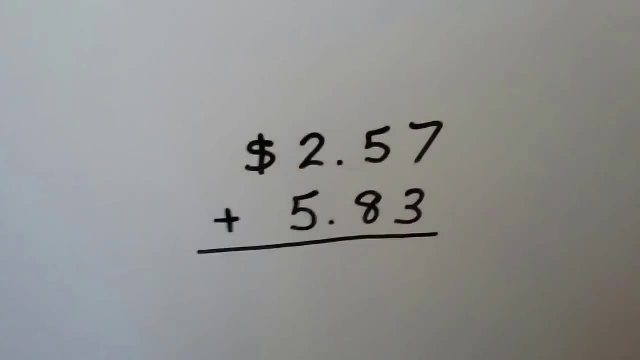 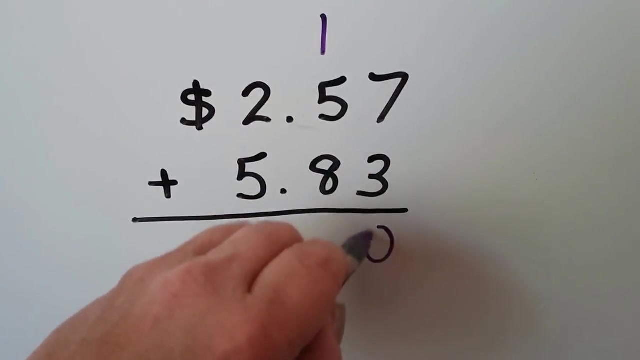 pretty column And we have: 6 plus 1 is 7.. We have $7.03.. All right, Let's try one more addition, one before we do subtraction. We have $2.57 and we're going to add $5.83.. We add the ones: 7 plus 3.. That's a 10.. We regroup the 1 and put the 0 down. Now we have to. 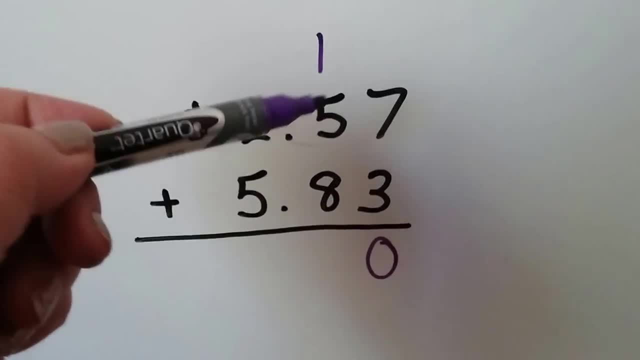 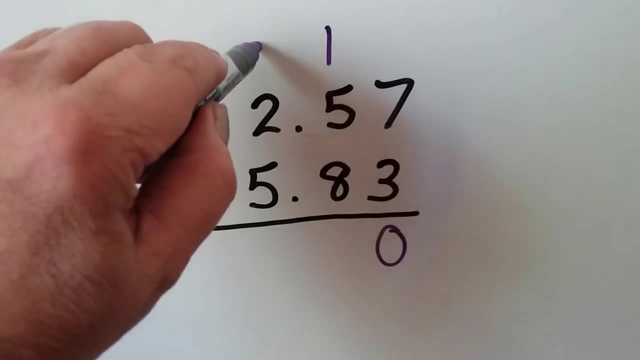 add the 10s place, We have 8 plus 5.. That's 8,, 9,, 10, 11,, 12,, 13 and one more is 14.. We need to regroup it as the 1 up here and the 4 down here. So now we gave 1 to the dollars, didn't we See our? 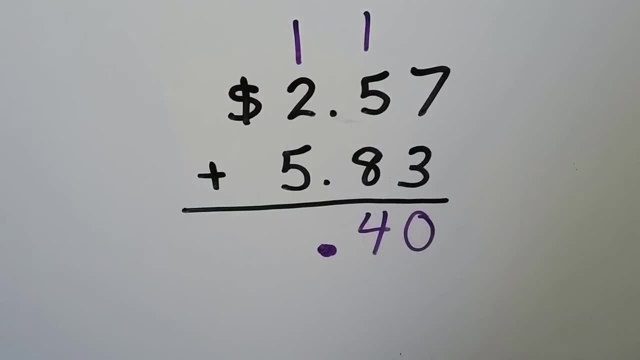 column coming down, We have $5.83.. We add the ones 7 plus 3.. That's a 10.. We regroup the 1 and put the 0 down for our decimal points. We need to put our decimal point there and add our dollars. We have. 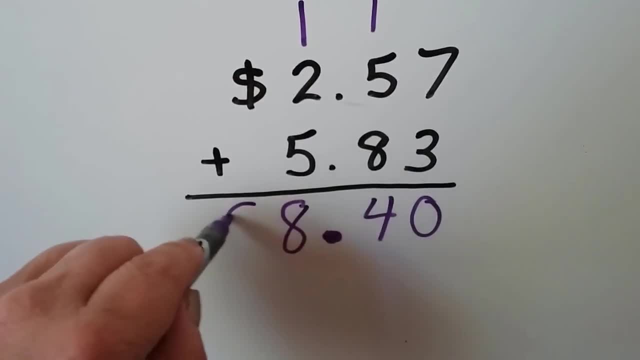 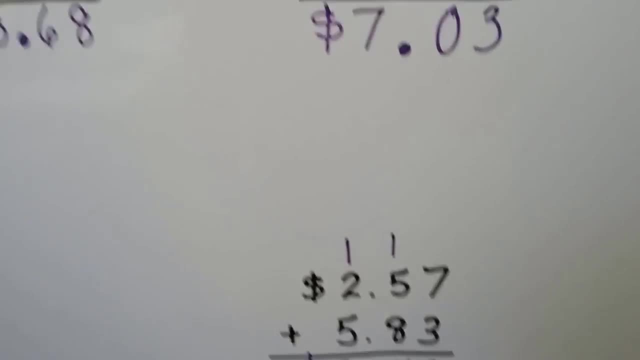 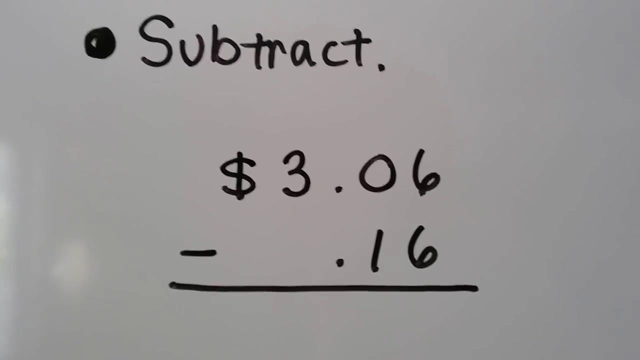 5,, 6,, 7, 8.. We have $8.40.. Okay, All right, Let's try some subtraction. We have $3.06 and we need to take away 16 cents. We start with the ones place and remember we might need to regroup. Okay, We're. 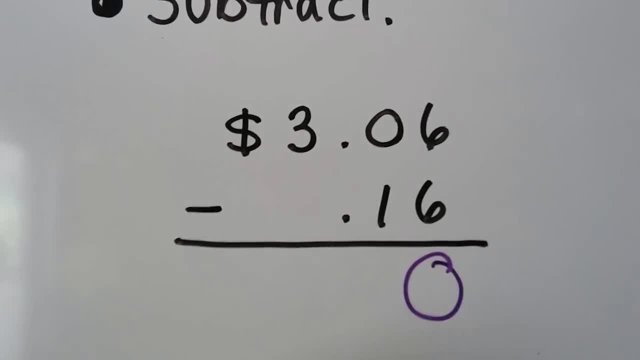 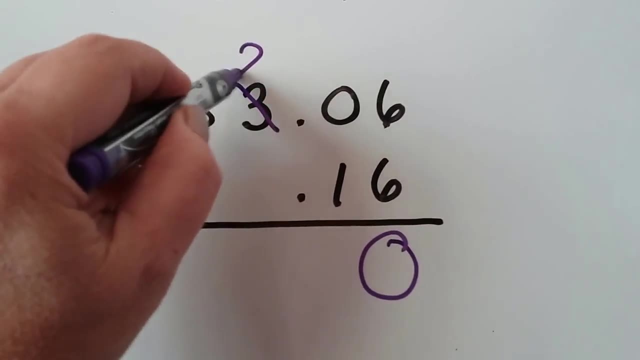 going to take away 6.. Take away 6.. That gives us a 0, doesn't it 0? take away 1.. Well, we can't do that. We need to borrow from the dollars. It's going to become $2 and this is going to become. 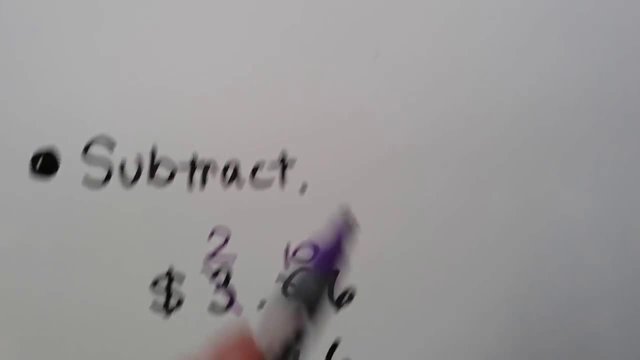 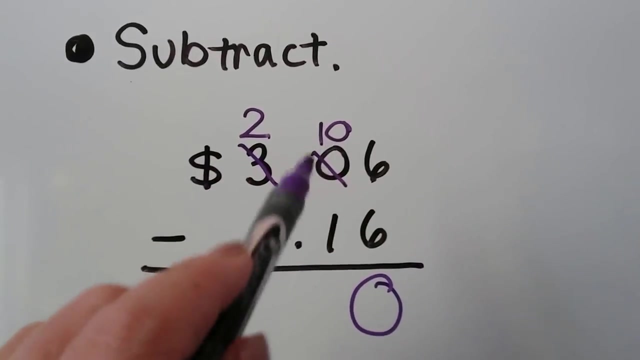 10 tens because 10 tens are equal to a dollar, aren't they? So if we take one of the dollars away from here and give it to the tens place, as 10 tens, that's the same thing as that dollar. Now we can have 10 tens and take away 1 ten. That's going to give us 9 tens. 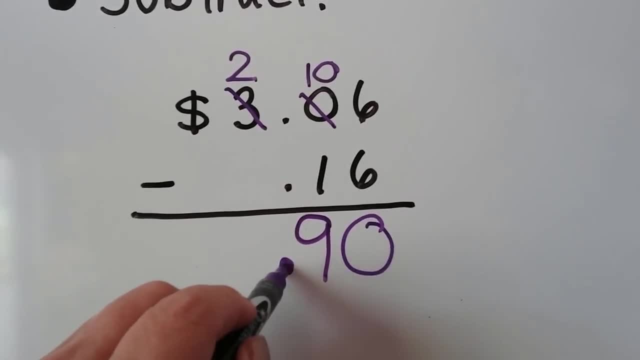 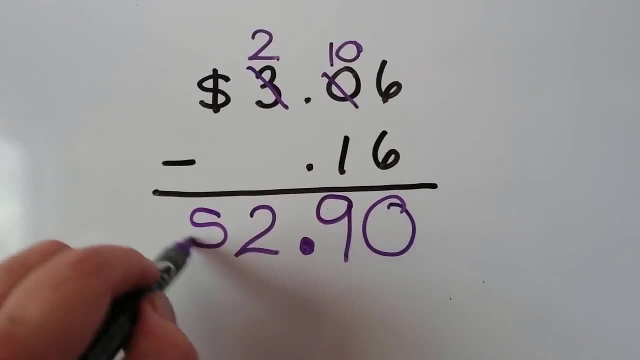 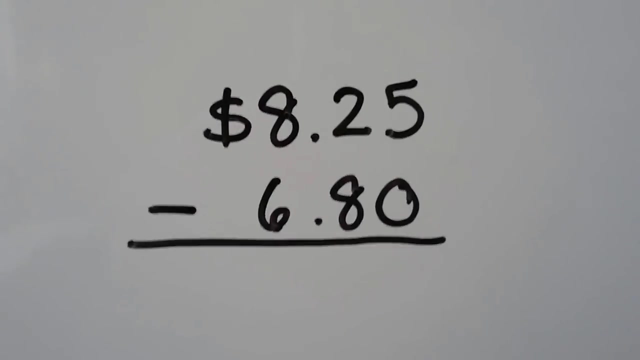 We remember our decimal point in a nice straight column and we bring down the two because we're not subtracting any other dollars from it, and we remember our dollar sign. We have two dollars and ninety cents. Let's try another one. We have eight dollars and twenty-five cents and we're going to. 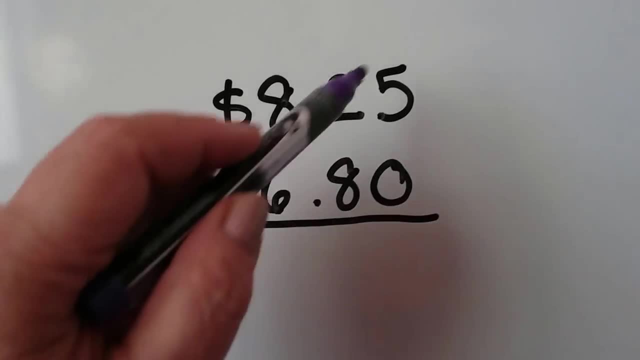 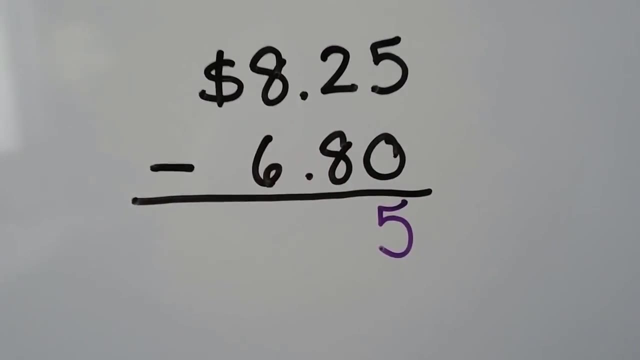 take away six dollars and eighty cents. We do the ones place first Five minus zero. Well, that's easy, That's a five. We have two and need to take eight away. We can't do that, so we're going to have to. 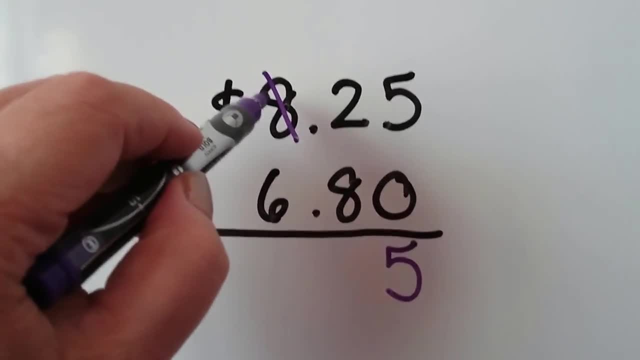 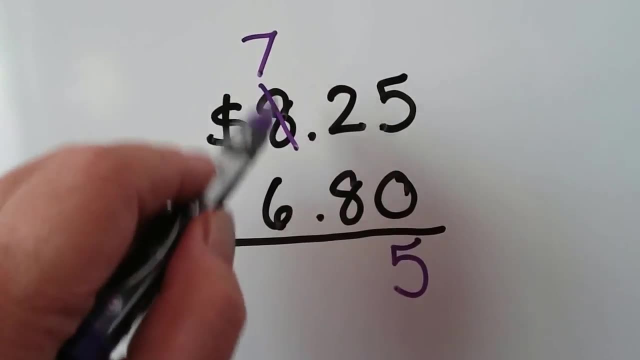 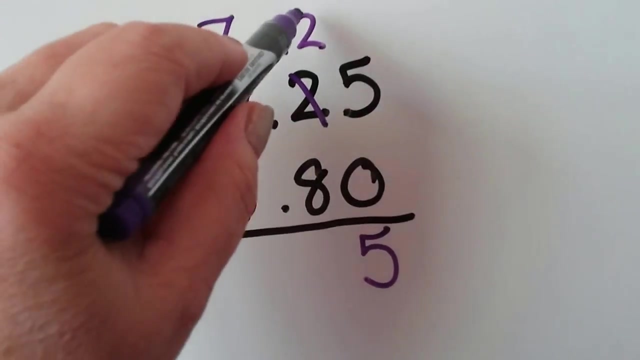 borrow from the dollars, aren't we Eight? Can we have a dollar? He says yes, He becomes a seven. This two becomes a twelve, because we're taking ten tens, which is a dollar, and we need to regroup it. Now we have twelve, take away eight and that gives us a four. 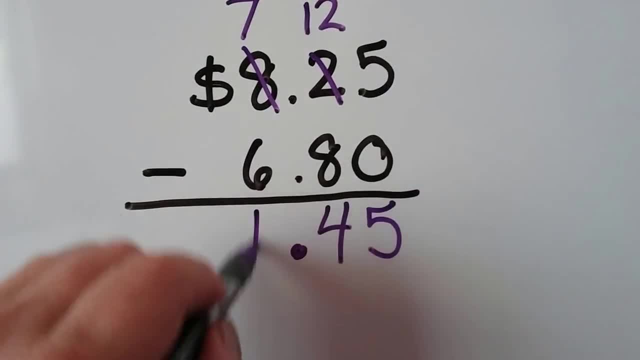 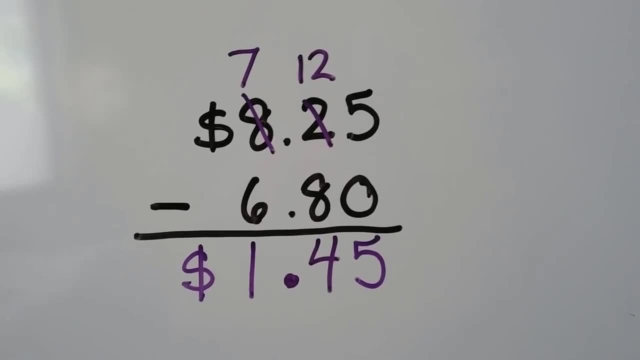 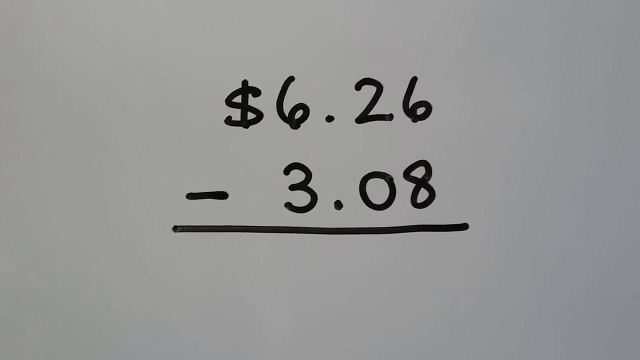 Remember our decimal point: Seven, take away six is one, and we have one dollar and forty-five cents for our answer, for our difference. Okay, let's try one more. We have six dollars and twenty-six cents. We're going to take away three dollars and eight cents. We start with the ones. Can we have six cents and take eight? 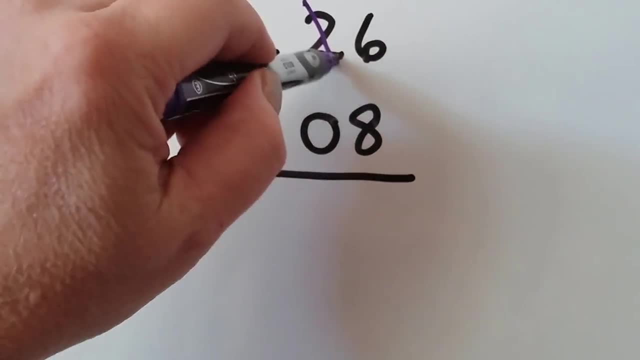 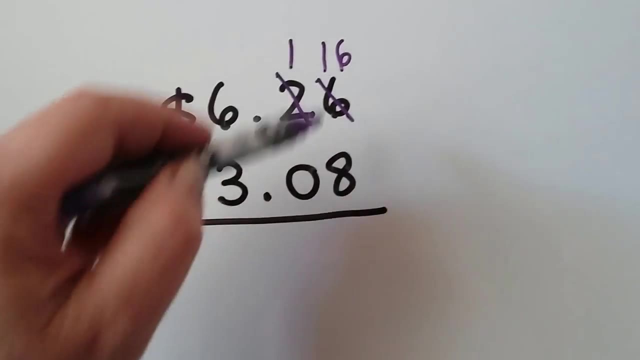 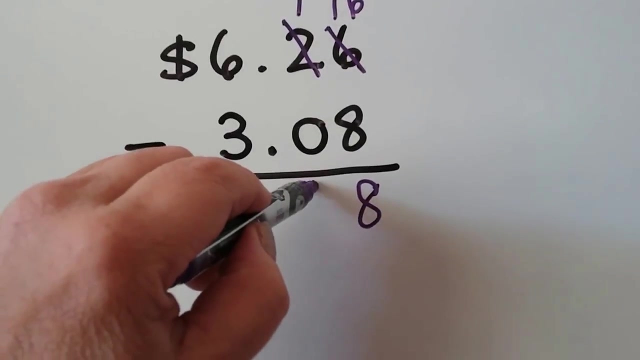 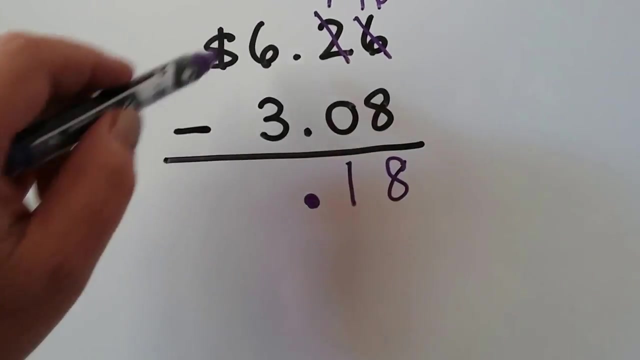 cents away, Nope. So we need to regroup the tens as one ten, and this is going to be a one. This one is going to become sixteen ones. Now we have sixteen, take away eight, That's an eight. We have one, take a way zero, That's going to stay a one. We bring down our decimal point, nice, in a straight column and we 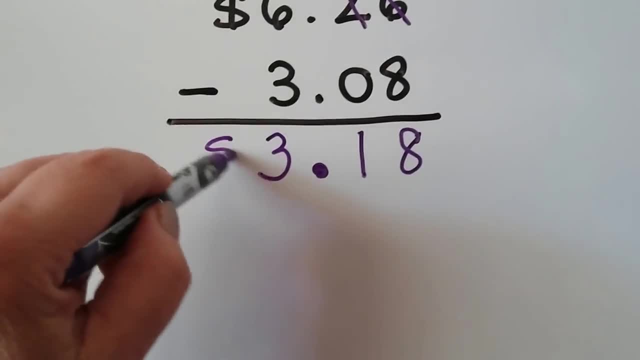 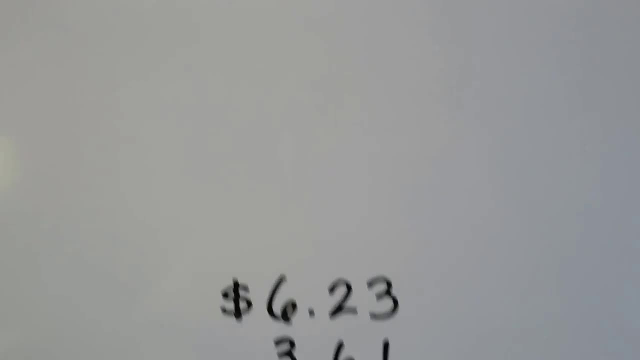 do six minus three, which is three. Remember our dollar sign. We have three dollars and eighty-seven cents for our difference. Try another one. Let's pretend, Let's pretend, Let's pretend, pretend. this is how much money we have when we walk into the store and this is how much. 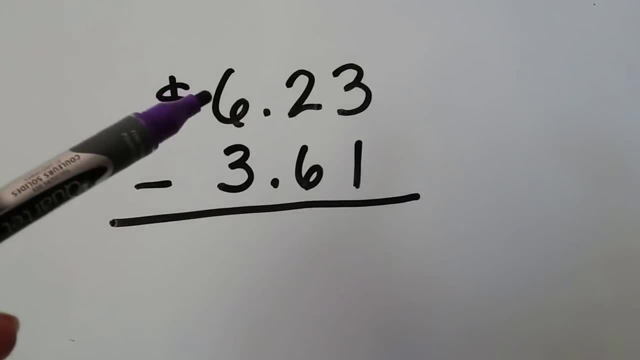 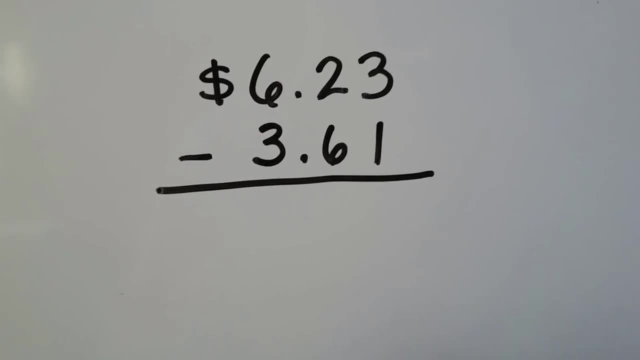 we're spending. okay. So we had $6.23, and we're going to spend $3.61, and we want to see how much we have left over. okay, So let's start with the ones. Three take away. one is two. Two take away. 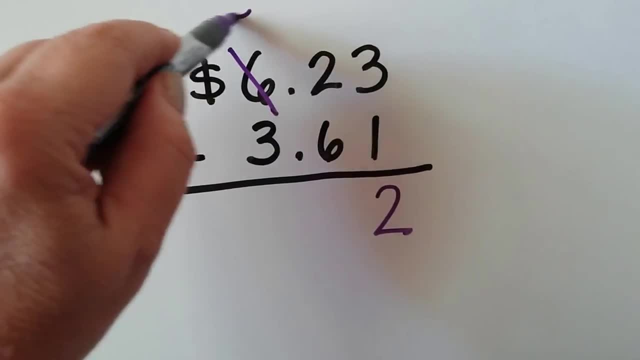 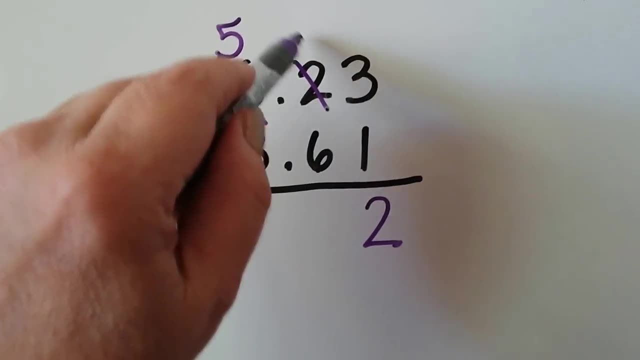 six Got to regroup. That's going to become a five, and we're going to add 10 tens to this. So we're going to add a 10 to that two. So that's going to become a 12 tens, isn't it 12, take away.